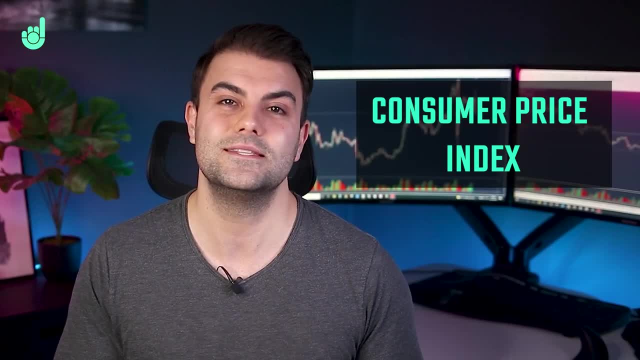 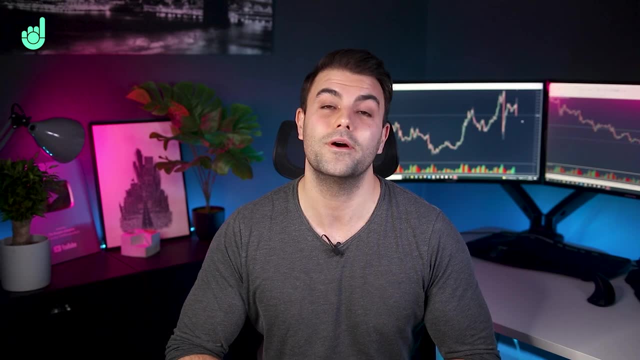 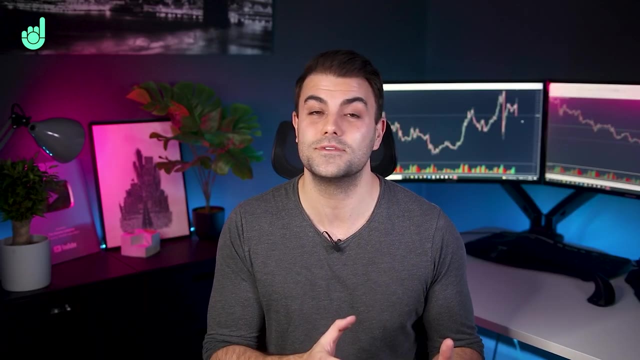 even makes it onto the mainstream news. It's the Consumer Price Index, also known as CPI, which is a measure of inflation. So let's start off by briefly going through what inflation is. Individual prices of goods and services will change over time in the economy. 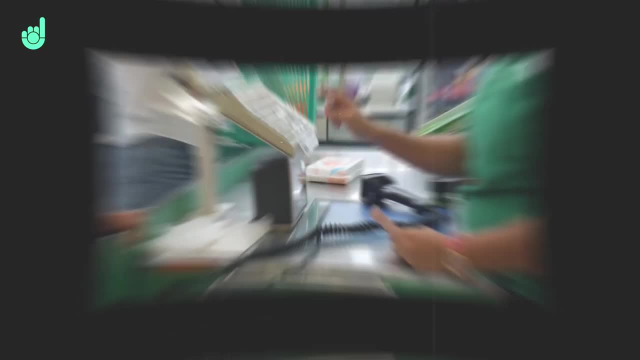 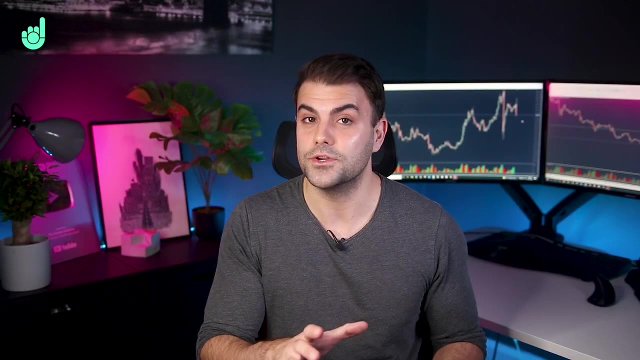 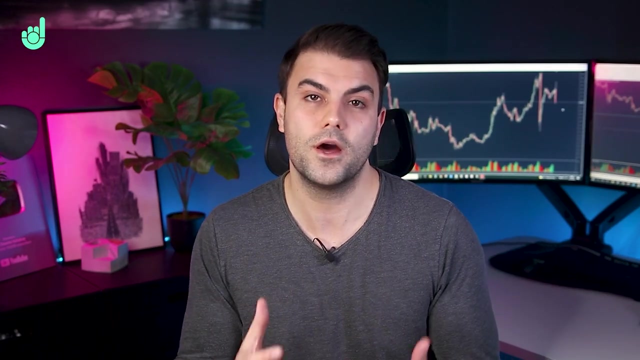 Some things will go up in price, some things will go down in price, but collectively the general price level in the economy will either be rising or falling. So inflation refers to a rise in the general level of prices of goods and services in the economy. This also means that the purchasing 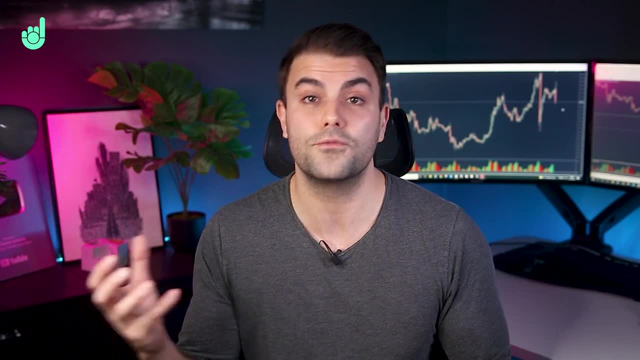 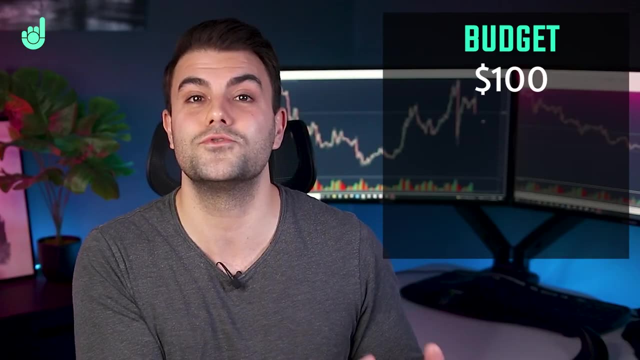 power of the currency is reduced, since a unit of currency can now buy less than it could before. If you try to buy every single item in the market, that's a lot of money. For example, let's say that you have a weekly shopping budget of 100 dollars and, in 2020, everything on your 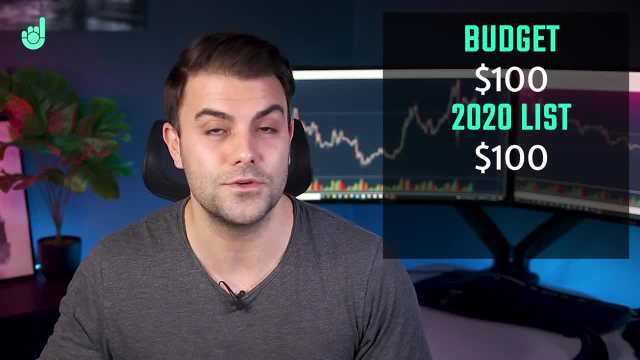 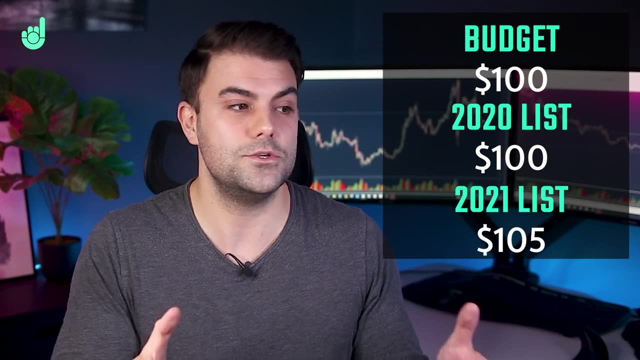 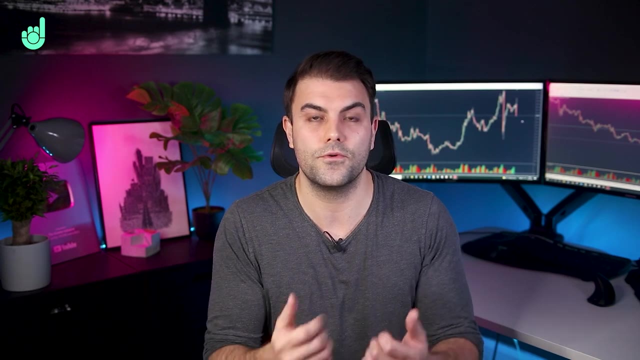 shopping list cost you exactly 100 dollars. What are the chances, However, one year later, in 2021, those same items on your shopping list now come to 105 dollars. So this means you can either not buy as much as you could before, or you have to pay more money to get the same items. In other words, 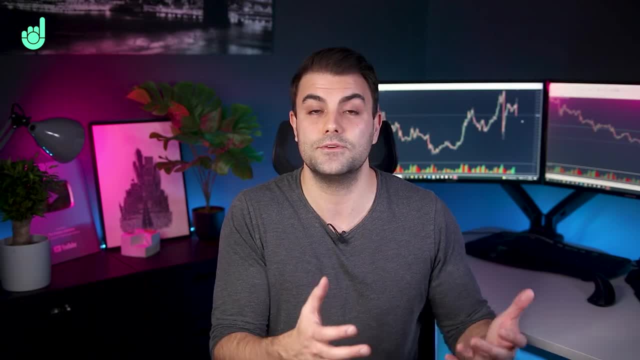 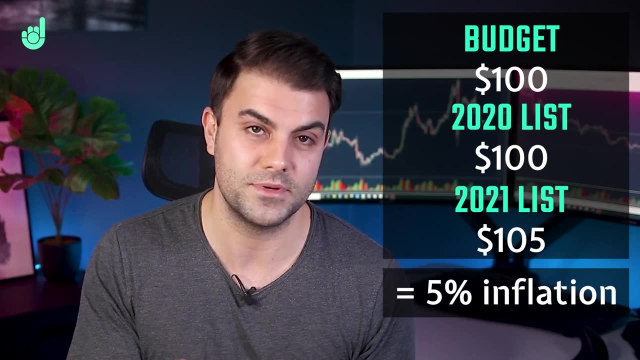 the value of your money has decreased. If that runs low, they're speculating that a direct rise in the, that rise of the price of your shopping list, is representative of what's going on in the entire economy. we would say that year-on-year inflation in the economy has risen by five percent Now there. 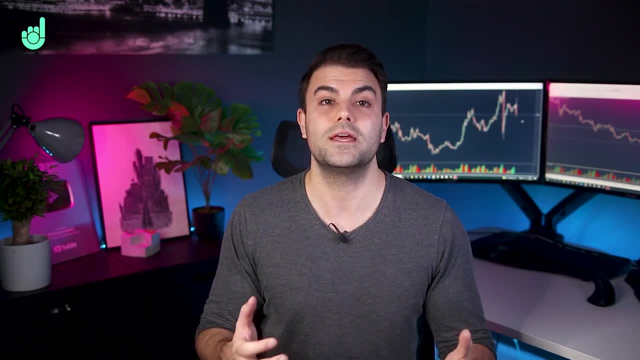 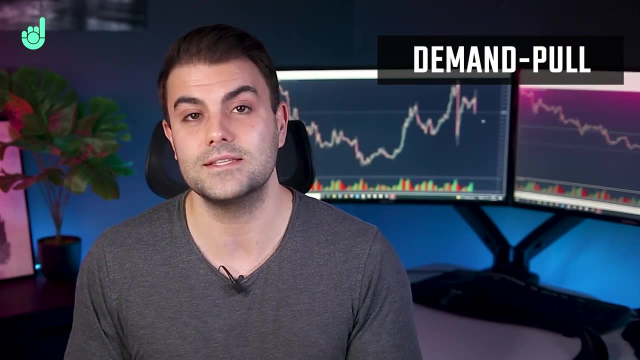 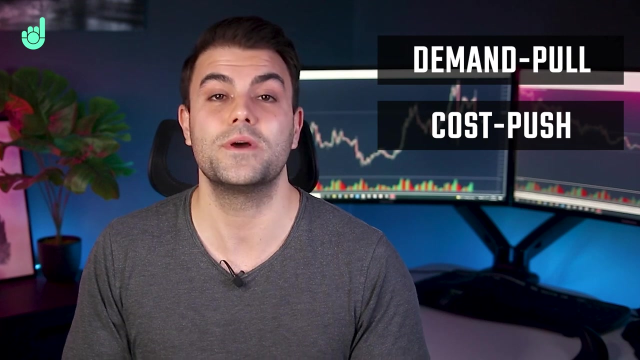 are many different factors that can influence inflation, but generally we refer to three broad categories of inflation. We have demand pool inflation, which means that prices are rising because there's more demand- more demand than the supply for goods and services. We have cost push inflation, which is when the cost of producing goods and services is higher, perhaps due to the 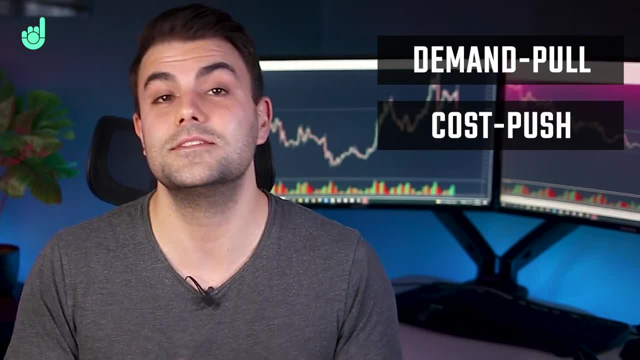 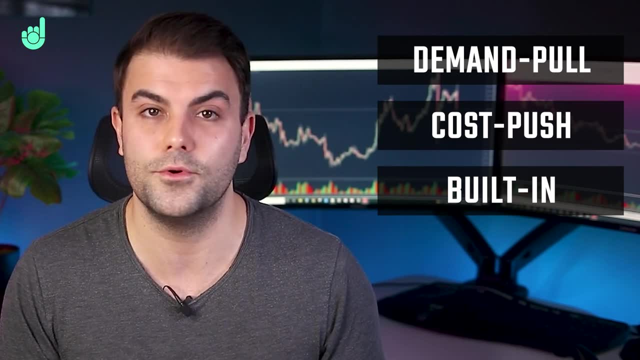 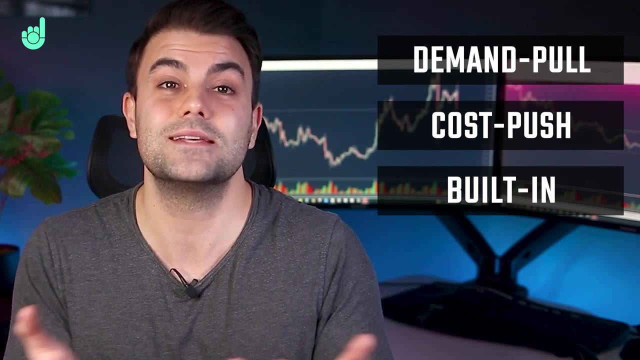 cost of wages or materials that are increasing in price and built-in inflation is when cost push or demand pool. inflation sticks around for a while and becomes a normal and expected aspect of the economy, which leads to things like people demanding higher wages, which then leads to prices. 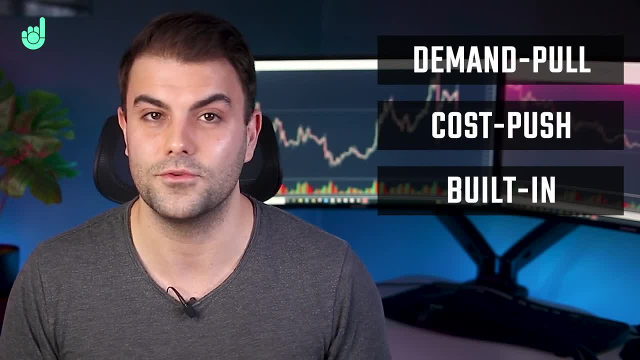 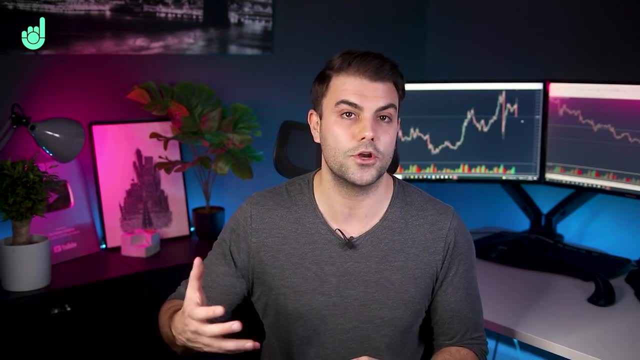 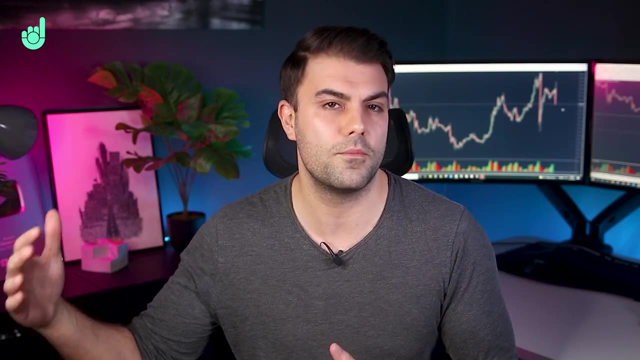 having to rise to account for that and leads to this wage price spiral. So inflation is expected when an economy is growing growing. So some inflation can be a good thing because it shows the economy is doing quite well. Most major central banks target a 2% inflation rate, but if it pushes too far above that or too, 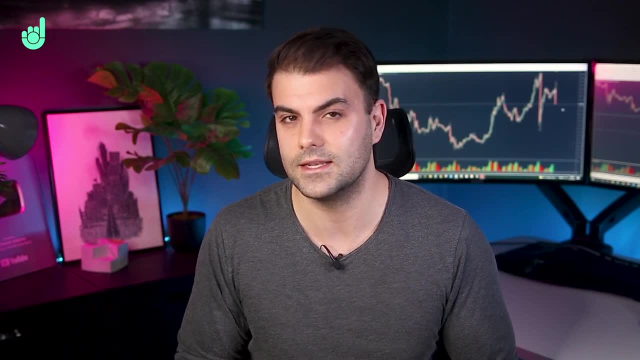 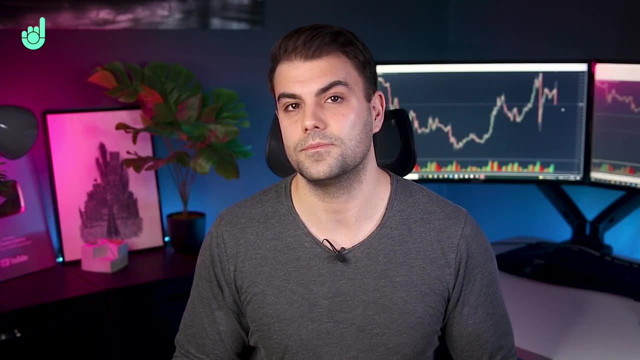 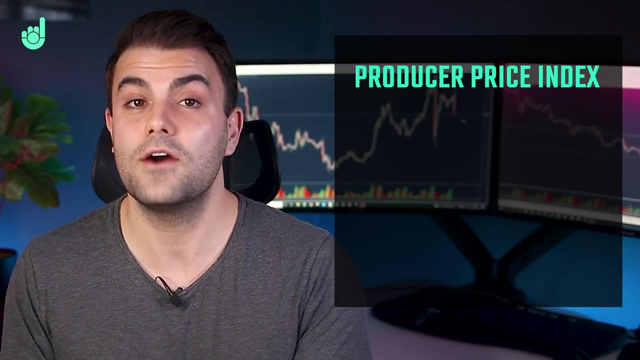 far below that, they may have to take action. We'll discuss that in a little while. Now, there are a number of different ways to measure inflation. Three of the most popular ones are the producer price index, which measures inflation at the production stage. Then we have 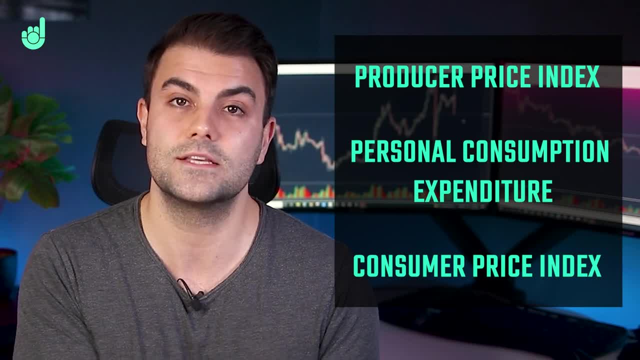 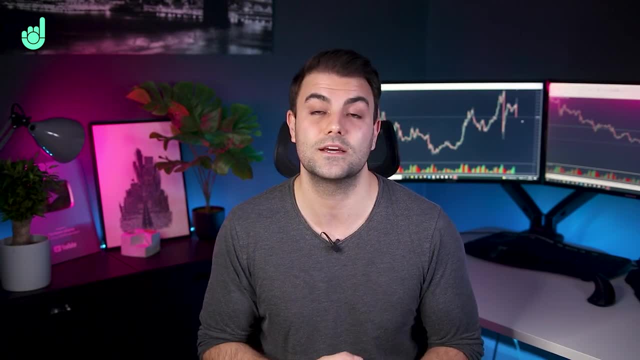 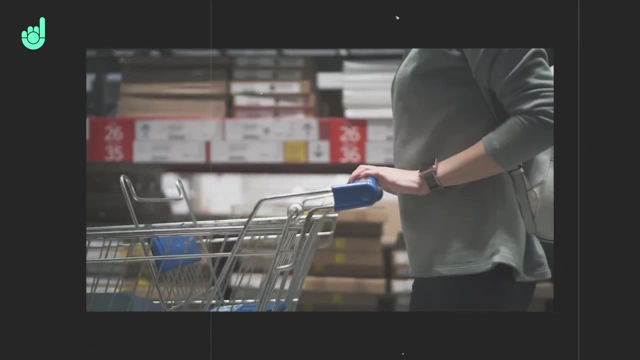 personal consumption expenditure and the consumer price index, which both measure inflation for consumers. So CPI is a monthly release that measures the change in prices that consumers pay for a basket of goods. Similar to that example I gave a bit earlier about the shopping list, CPI usually includes goods that are regularly purchased by households, such as food, energy. 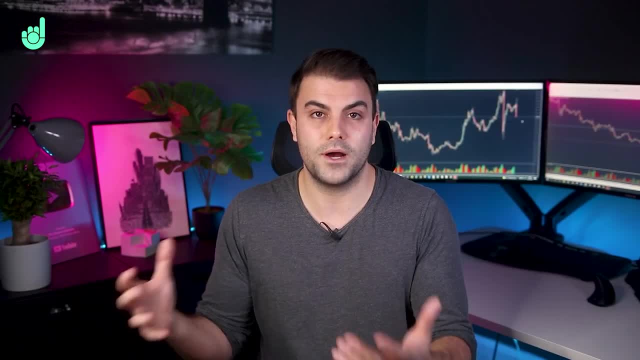 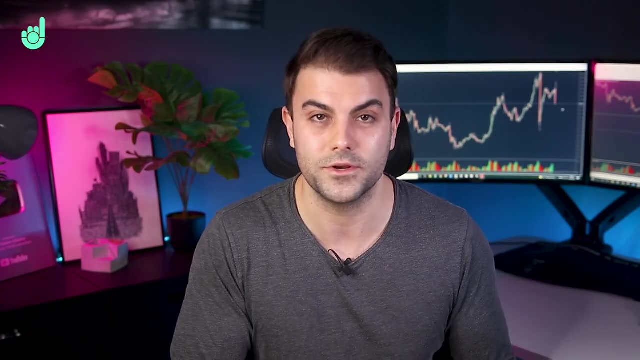 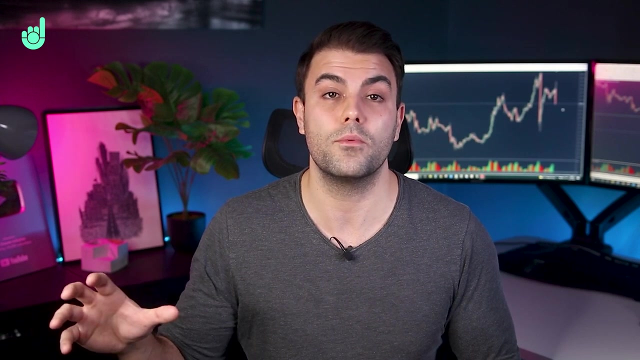 furniture and so on. However, what's included in that basket of goods will vary depending on the country. Now, this basket of goods doesn't include every single item we could all possibly buy, since that would really be impossible to collect regularly, So instead it sort of represents a sample of what we call. 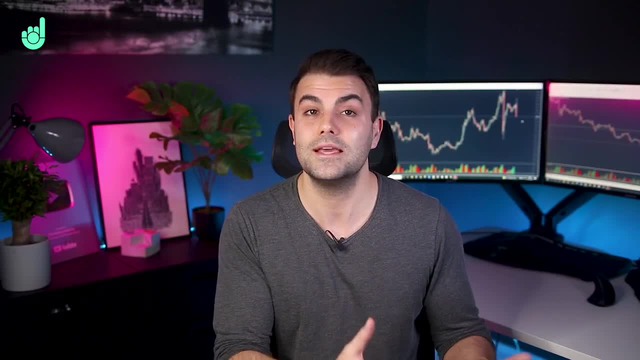 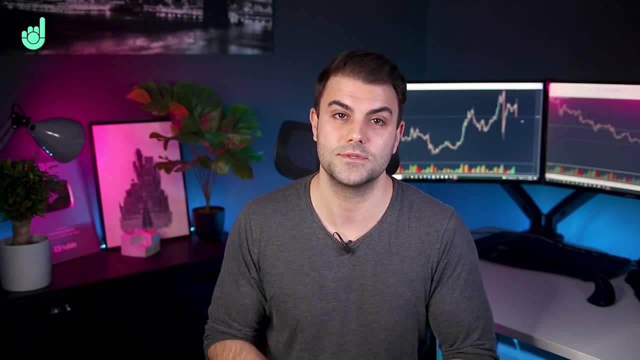 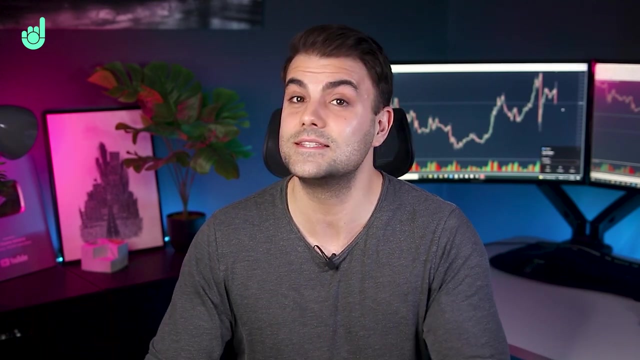 representative items. For example, in the UK CPI release there are 700 separate items and over 100,000 prices are collected for those items. Now some people assume that CPI is for essential items or it's a gauge of the cost of living, but that's not necessarily the case. For example, the UK 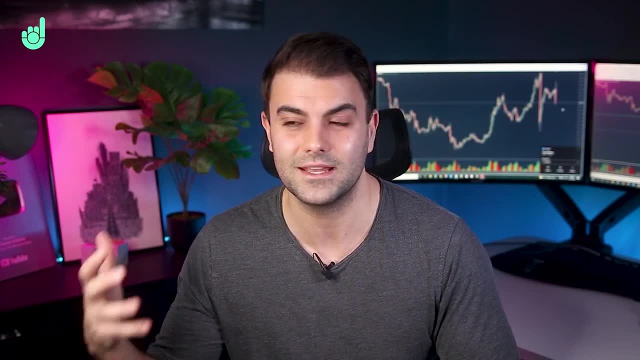 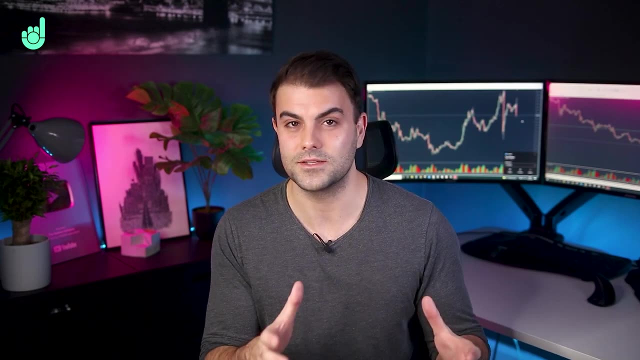 their release includes the price of cigarettes, which isn't really an essential item for most people- at least it's not for me, maybe in the past. Now the index is a weighted average of this basket of goods, So what that means is that each item that's included has a different weighting. 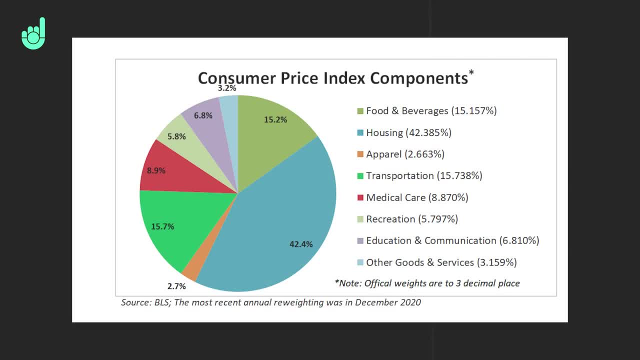 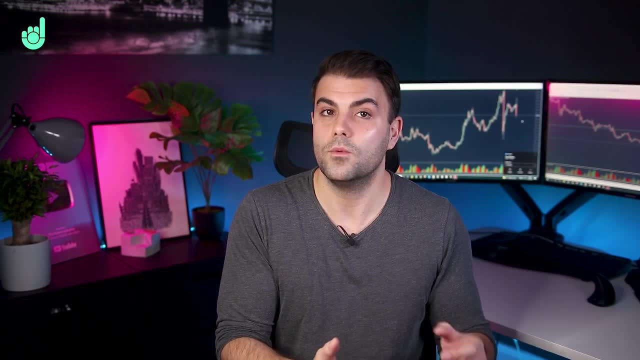 based on how important that particular item is, So in other words, like what share of total household consumption that item accounts for. So price rises of each item will affect the index differently, based on what their weighting is, Something that has to do with the price of the 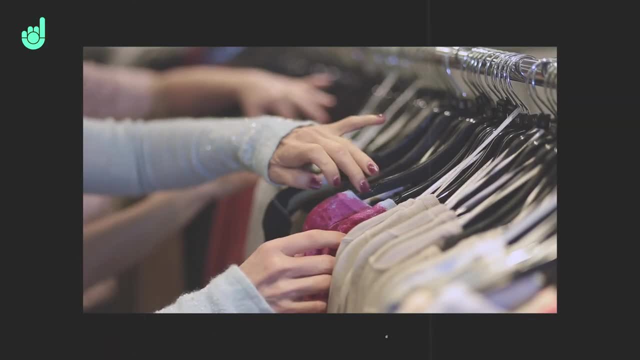 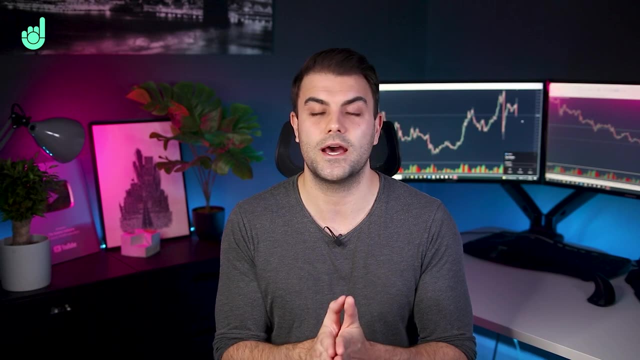 product is a higher weighting will affect the index more than an item that has a lower weighting, So it's weighted more towards these important items. The release shows us the percentage change for a period of time, typically monthly or yearly, And it's usually also split between CPI covering. 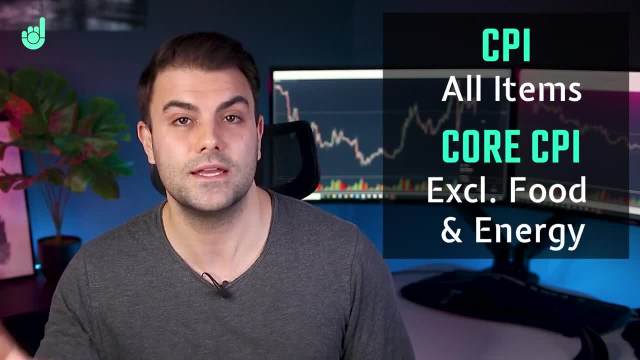 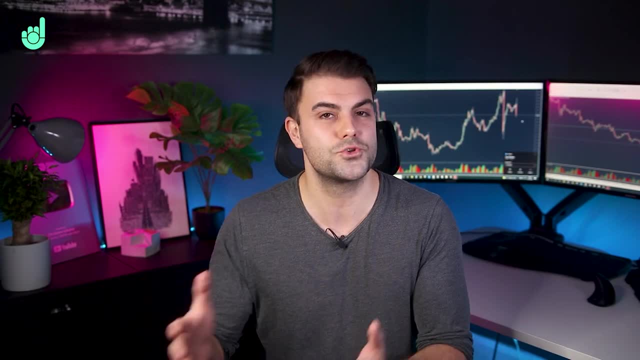 all items and core CPI, which doesn't include energy and food, since those items are usually more volatile. However, since households don't really have much choice but to buy those volatile goods, it's generally more important to look at the price of the items and the cost of the items. So the 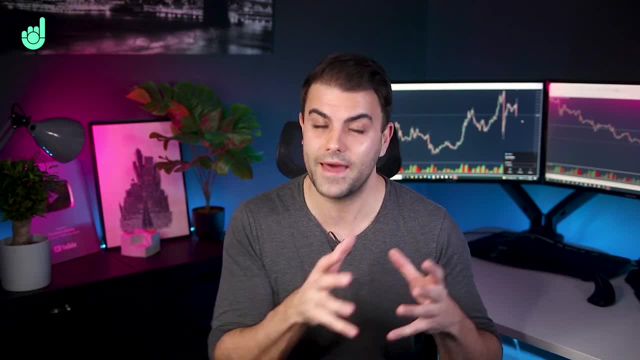 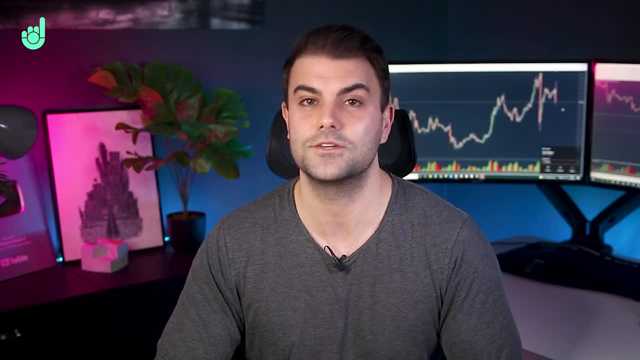 important to include them and that's typically why central banks favour that reading rather than looking at the core CPI reading. Now, some countries also choose to split the release into different categories. For example, the US. they split their release into CPI-U, which is for all urban consumers. 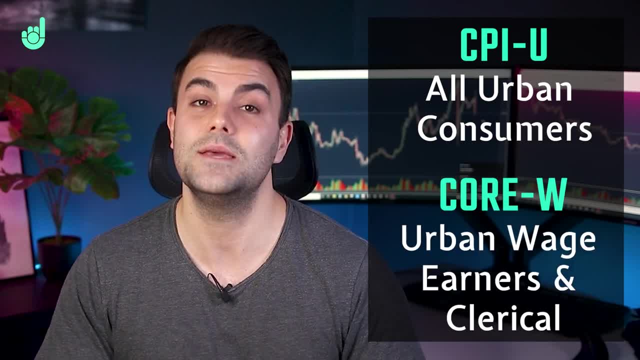 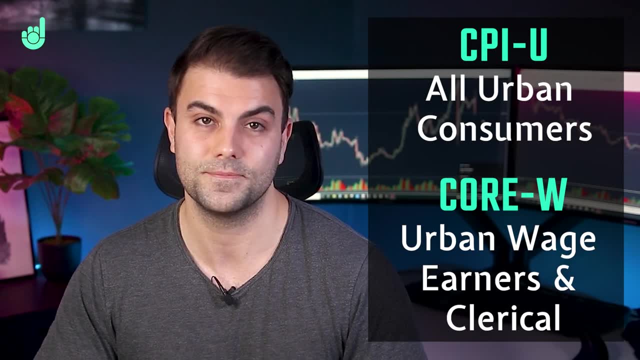 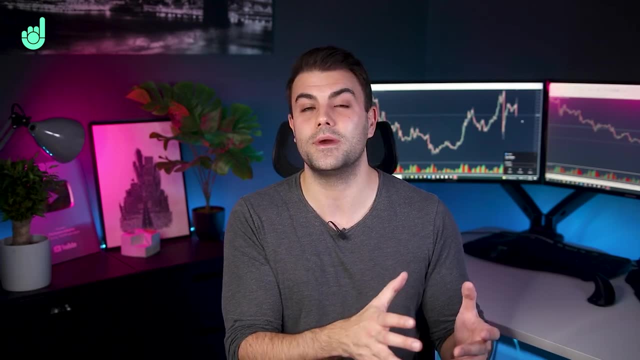 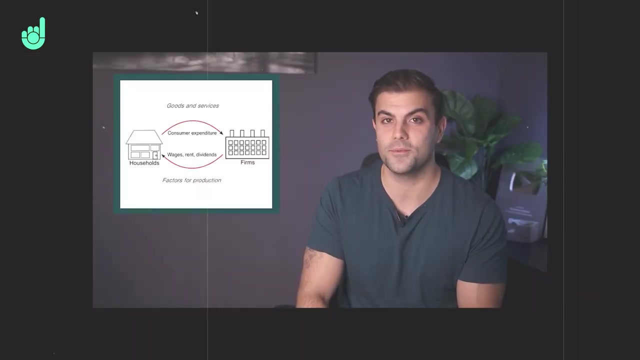 which represents 89% of the population, and CPI-W, which is for urban wage earners and clerical workers, which represents 28% of the population. Inflation, GDP and employment levels in an economy are all closely linked. If you saw our previous video about GDP, click up there to watch it. you'll remember that we discussed the inner flow in the 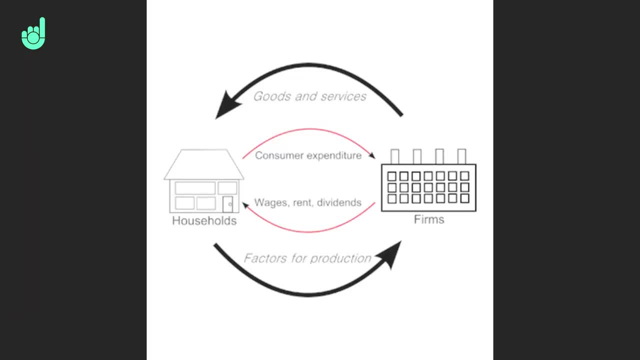 economy. So when more money is circulating in the inner flow, it means that companies employ more, people increase wages, which in turn means that consumers have more money to spend. so there's an increase in demand and, as we discussed earlier, this increase in demands can then lead to demand. 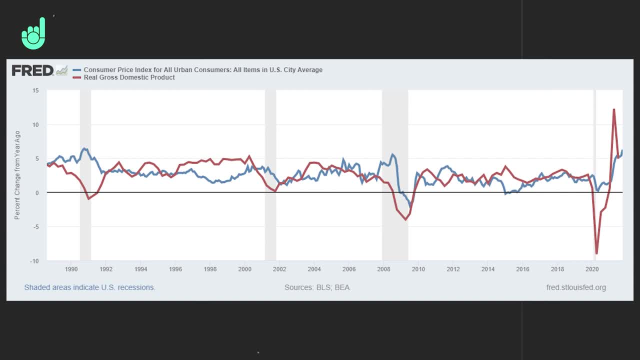 poor Inflation. so if inflation is on the rise, it can be a sign that an economy is growing. Likewise, if we look at employment figures, like the NFP release in the US, and see that wages are rising or the unemployment level is reducing, we can expect more spending in the economy as well. However, since too 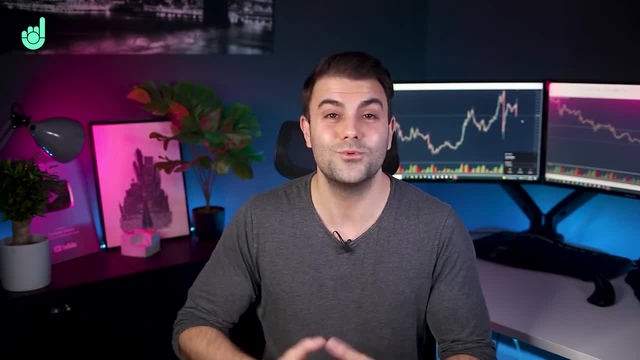 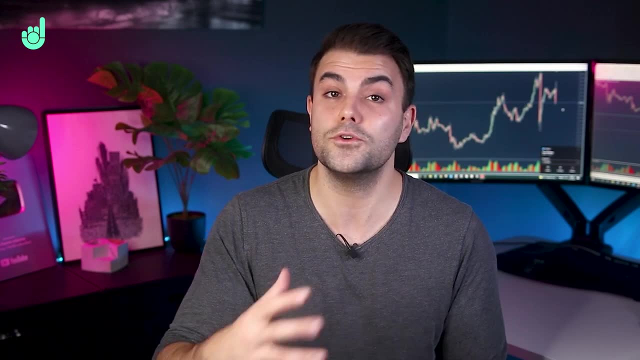 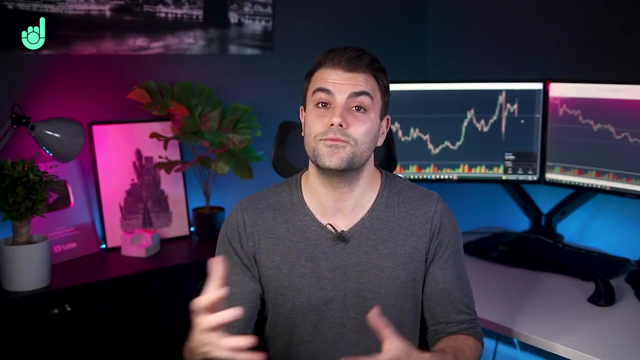 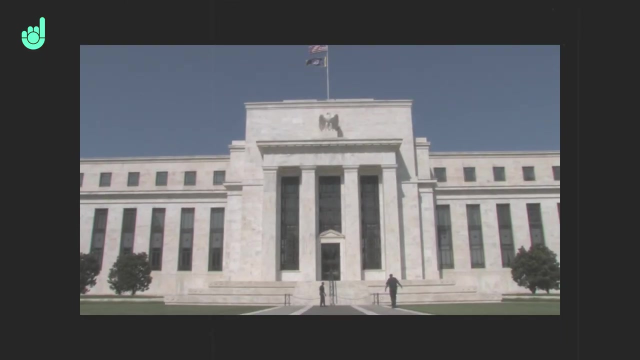 much inflation will be reducing people's purchasing power. it can also be harmful for an economy as well, especially if it gets out of control. This is where central banks come into the equation, as they'll usually be targeting a poor economy When inflation starts to rise too much. this is when central banks will start to look to take action. 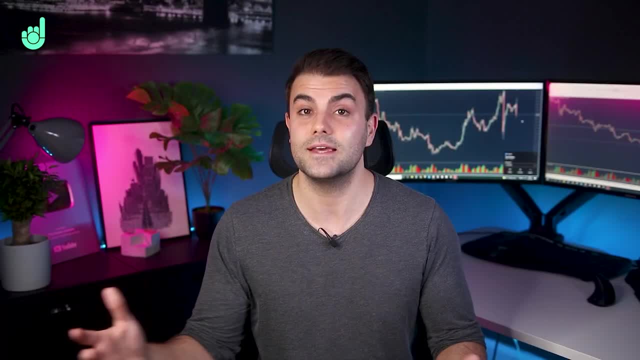 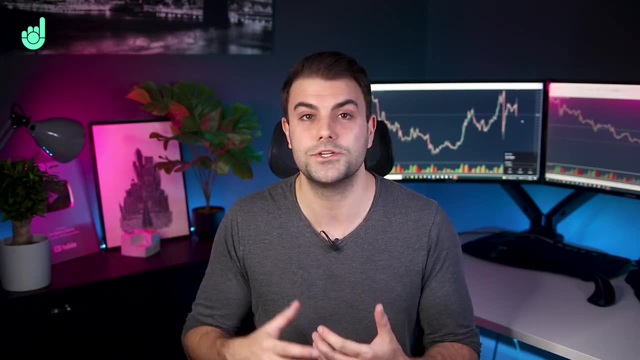 by doing things like raising interest rates. By doing this, they make it more expensive to borrow money and it incentivises saving money more, both of which will lead to a reduction in the level of money circulating in the economy. So this is why we see things like the dual mandate that the federal government has in the economy. It would cause spending to fall and therefore to inflation dropping. This means that central banks need to follow the economy's CPI data closely, along with other measures of inflation, to help make their decisions. It's also why the market follows it.